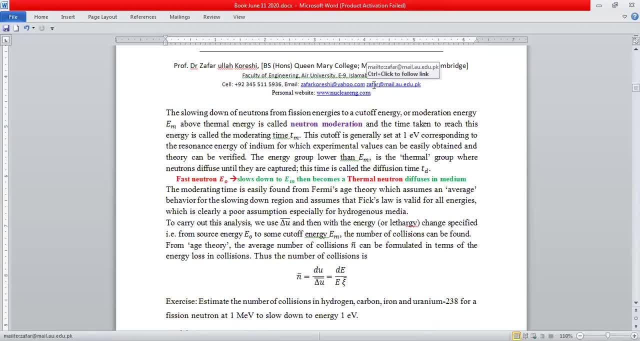 and official address is zafarauedupk. my cell number is 923455115936 and personal website is wwwnuclearengcom, So you're most welcome to send me your podcasts, Thank you. Thank you, points, suggestions, questions. I'll be really happy to answer anything that you'd like me to. 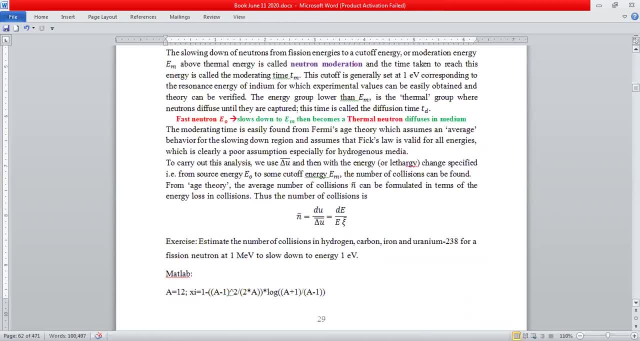 answer. Okay, so let's continue from the previous lecture. So we're looking at the slowing down of neutrons. Now. the slowing down of neutrons, let's start at a high energy, like efficient energy, And let's say that it comes down from efficient energy, which is typically. 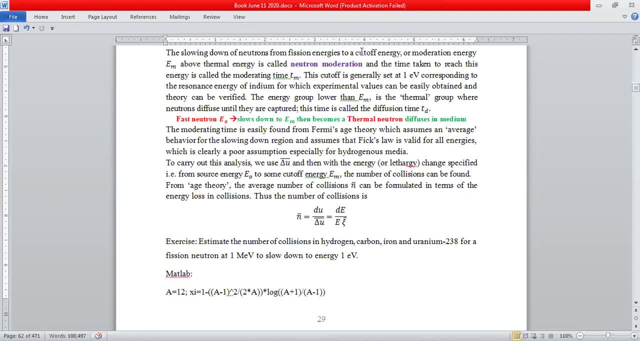 one to two MeV. it comes down to some cutoff energy and or some moderation energy, EM. let's call it EM- which is above thermal energy. So the slowing down process, the moderation process, is called neutron moderation And we'll try to see what we can. 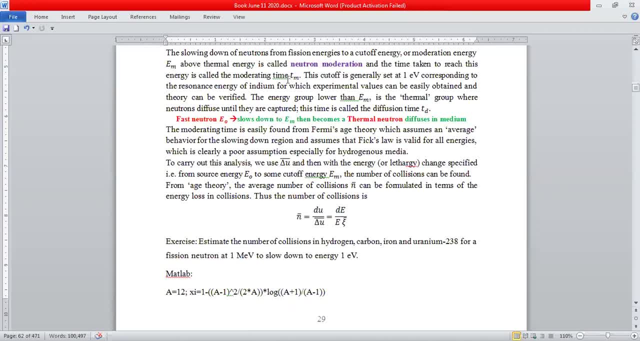 get about this And how much time does it take to reach such a low energy, such a low cutoff energy? Now, this cutoff energy cutoff is typically set to one electron volts, So you're dealing with one MeV approximately, down to about one EV. So that's six orders of magnitude, And in between you've got resonances. So 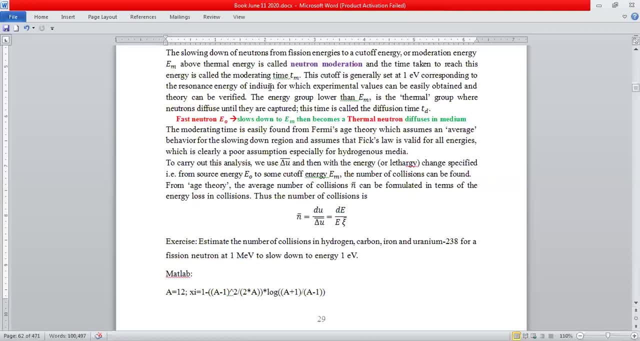 experimentally. what's done is that you put in a material inside a nuclear reactor, such as indium. it has a resonance energy for which experimental values can be easily obtained and we can verify the theory. Now, energy lower than the moderation energy, EM, is called the thermal energy. So in your mind, 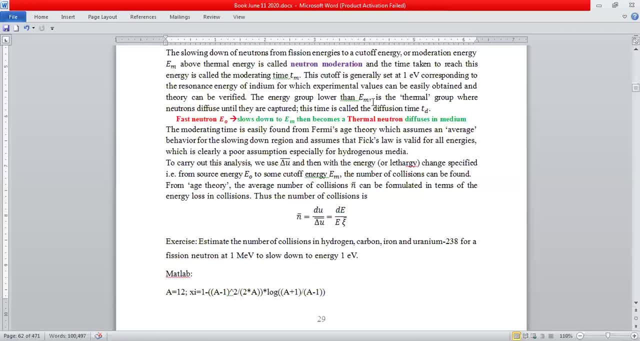 you can essentially have two separate compartments: one slowing down from MeV to EV, The second once you come down to EV. so one EV down to 0.025 EV. So the first thing you call slowing down or moderation, The second, once you come down to EV, so one EV down to 0.025 EV. 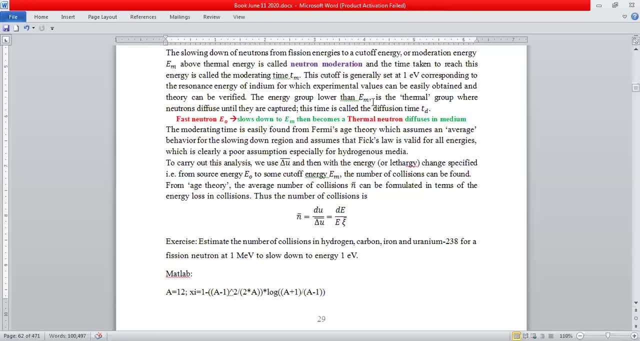 The third thing you call diffusion. And when it diffuses, it's captured, it finishes, it strikes, so that time is called diffusion time. So we've got a moderating time, TM, and we've got a diffusion time, TD. So in red and green- again I've written this down- Colors can be effective, that a fast neutron. 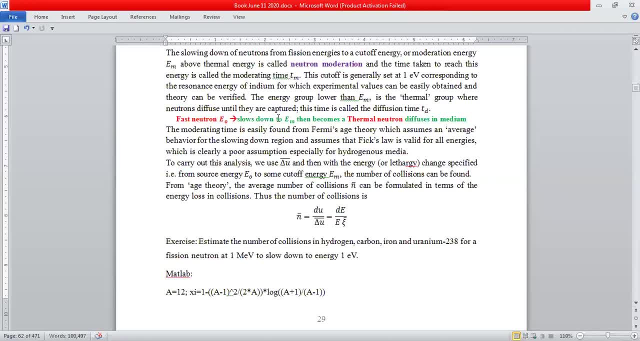 is born and some energy E naught. it slows down to some moderation energy Em. then it further diffuses, it becomes a thermal neutron. So here it's a fast neutron and here his name is a thermal neutron and he carries on diffusing inside the medium. 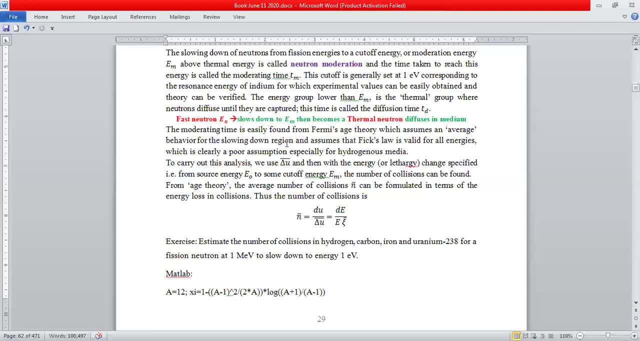 until it's captured or it leaks out of the boundaries. So the moderating time is easily found from Enrico Fermi's age theory. Now, this age theory, Enrico Fermi, I think his brilliance, his simplicity was that he made simple, simple assumptions. So he assumed that every neutron behaves like an average neutron, In other words, it gains an average amount of lethargy per collision. He also assumed that Fick's law is valid for all energies. Of course that's a poor assumption. 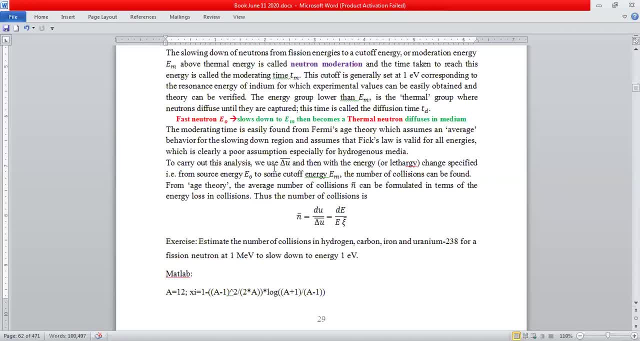 especially for a hydrogenous medium. Now he carried out his analysis further. He said that the number of collisions is a continuous variable and he used the average lethargy increase per collision from source energy down to some cutoff moderation energy to find the number of collisions which took place. 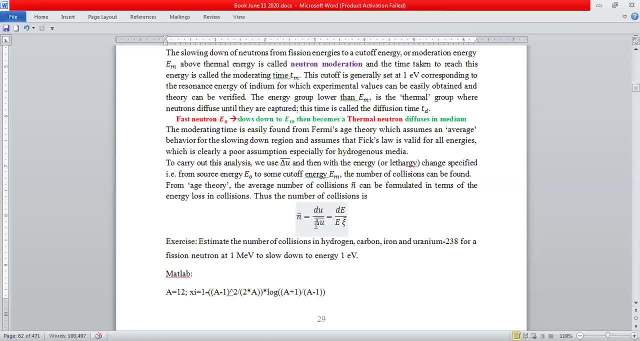 So N is how much you lose. divide by how much you lose per collision and it gives you the number of collisions that have taken place. So if you put the things together, which we did in the previous, where we calculated the average lethargy increase per collision, 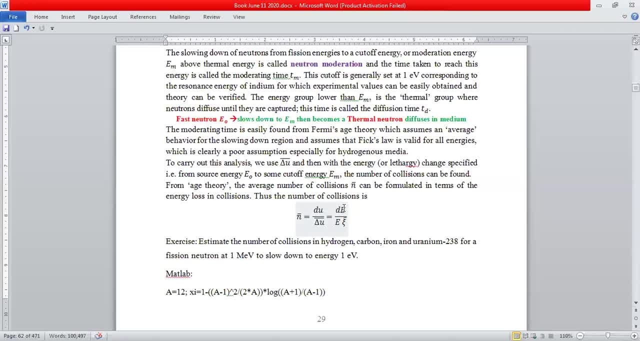 then you get that the number of collisions is dE over E And then the denominator. you've got a squiggle bar, which means that you can do it for mixtures or whatever you've got Now. I think it's very important for you. 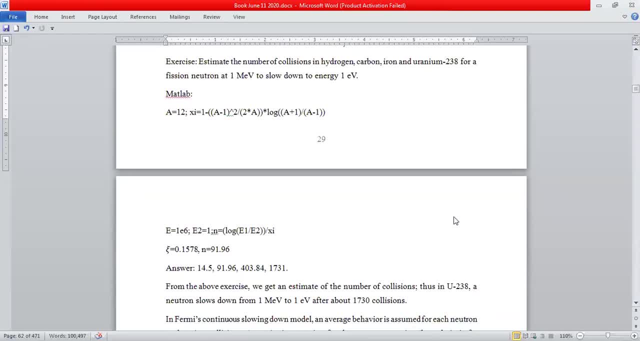 not just to look at equations and symbols but to go to MATLAB to put some numbers in there. So I've given you a little exercise that estimate the number of collisions a neutron undergoes when it collides with hydrogen carbon, iron, uranium-238. 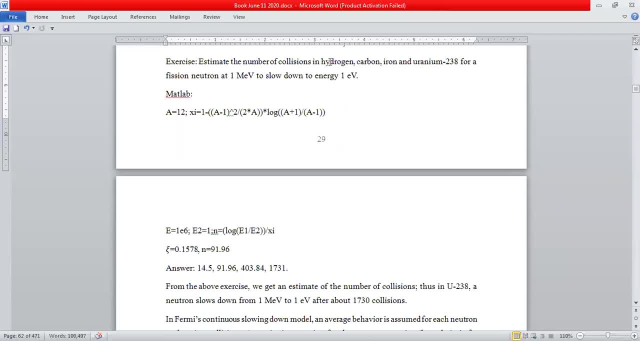 So these are the extremes of the periodic table: the lightest, the heaviest and things in between. Now, carbon is so important for us. in nuclear engineering we call it graphite, and graphite is used a lot as a moderator. We use iron, a lot steel. 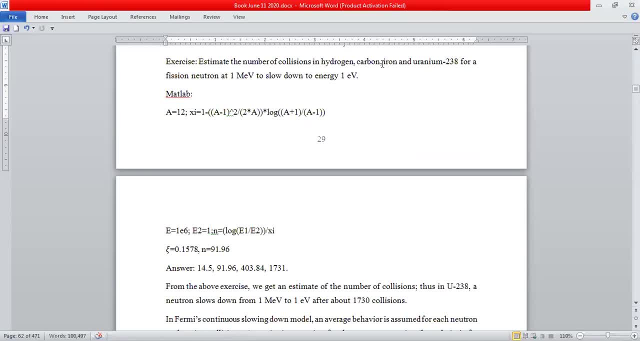 So steel is a structural material and vessels are pressure vessels, containment vessels. A lot of steel is used in engineering in industry. Hydrogen- so good, because alpha is zero. You can bring down a neutron from a high energy to a very low energy. you can thermalize it. 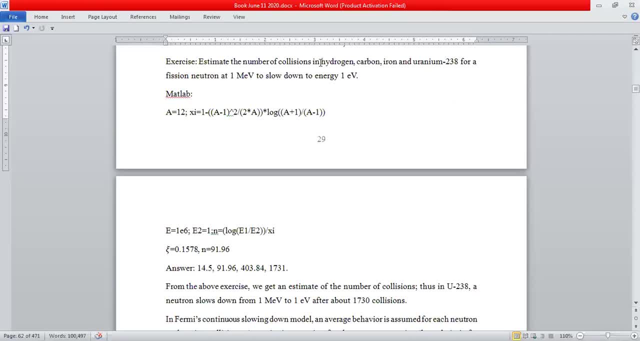 Why do you want to thermalize it? Have you thought that this is what we did in the first two, three lectures? Well, why do you want to? why is hydrogen so important? Because a neutron can be thermalized so easily. And let's see how easily can a neutron be thermalized? 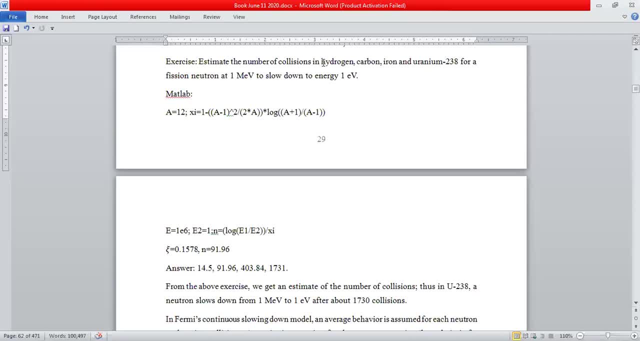 Why do you want to thermalize a neutron? Well, because the fission cross-section is very high at low energies. So how do neutrons behave in hydrogen carbon, iron and uranium-238? for a fission neutron which is slowing down from one MeV? 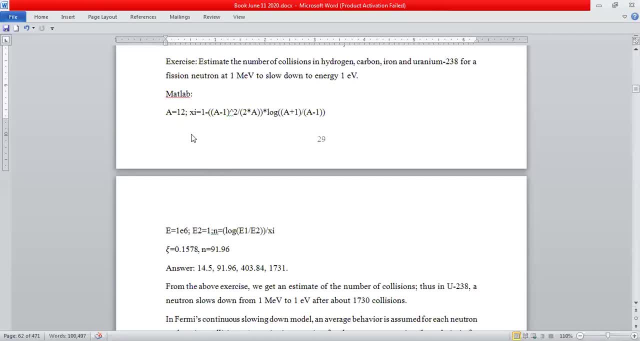 down to an energy of one MeV. So I just wrote these two lines in MATLAB. So for graphite, for carbon, A is 12.. You use the previous formula that psi is one minus 12. That's a minus one whole square over two A. 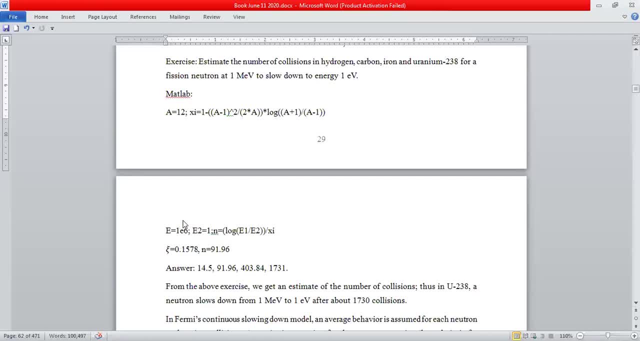 times log A plus one over A minus one. The initial energy is one MeV, The final energy is one MeV. The number of collisions is this. So that's the answer you get for graphite. So look at this. So in a single collision with graphite, 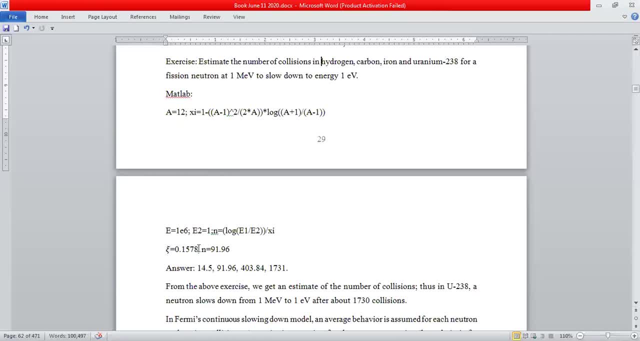 a neutron gains a lethargy of 0.1578.. Does lethargy have? has any unit? No, it doesn't. It's the natural log of E, naught over E. So U is, so E is yeah. 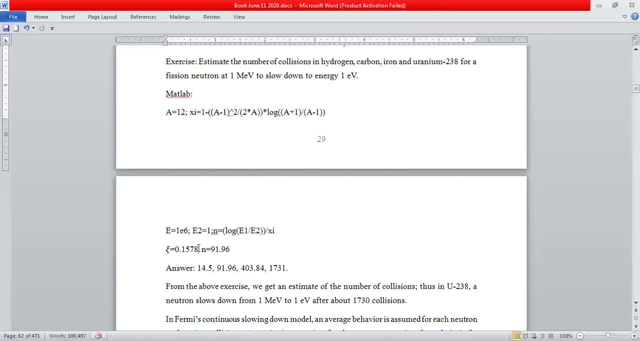 So E is E naught, E to the minus U. So if you take the logs on both sides so U is the natural log of E naught over E. So E naught is always greater than E. So that lethargy is always going to be a positive one. 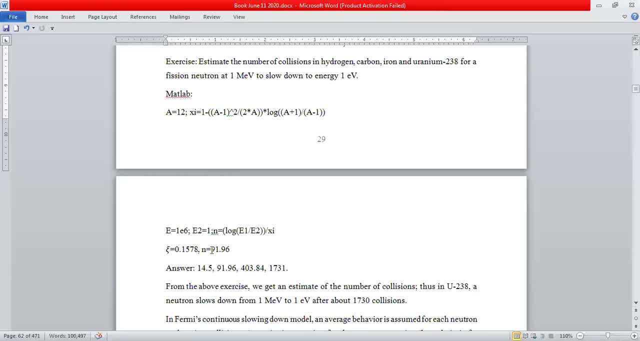 Now it takes about 92 collisions for a neutron in graphite To come down from one MeV to one E. So this is the first time that you are seeing a number to give you some idea of how many collisions take place to come down from a high energy. 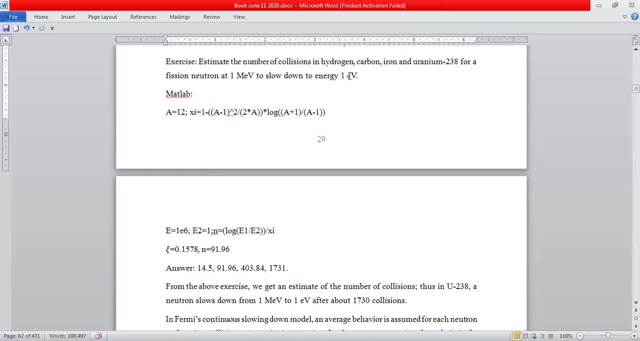 a fast energy to a slow energy. It's 92 collisions Now in hydrogen. it's about 15 collisions In graphite. as I said, 92 collisions In iron: 403.5.. 404 collisions In U238, 1,731 collisions. 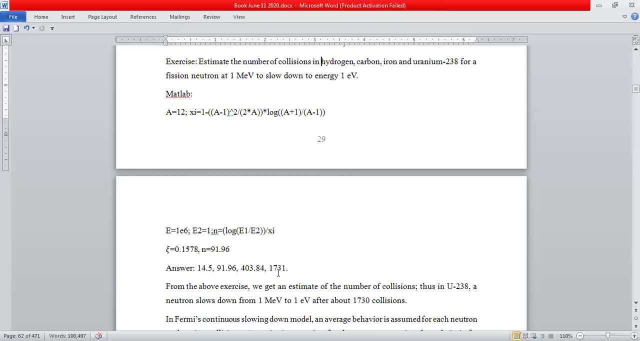 So how difficult is it? So would you like to slow neutrons by putting them in U238?? I don't think so. This is how you try to, so you try to use water. So, and yes, water is such a good moderator. 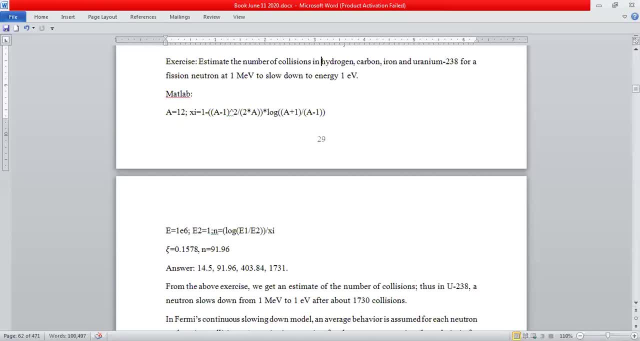 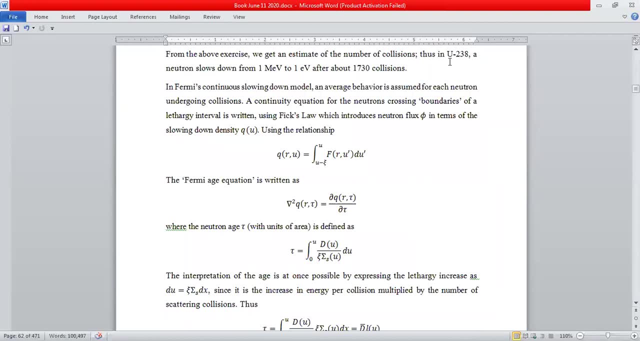 in nuclear reactors precisely for this reason. So from this exercise you get an estimate for the number of collisions. So from this exercise you get an estimate for the number of collisions. So you'd say that in U238, it took 1,730 collisions. 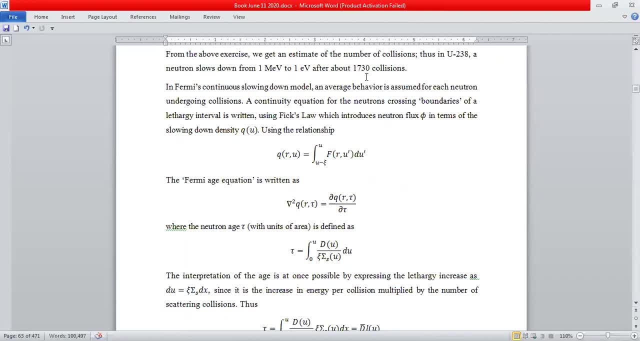 So U238 is a very bad material to thermalize a fast neutron. Okay, So that's the engineering deduction. Now let's go to Enrico Fermi. Enrico Fermi's continuous slowing down model. It's called the continuous slowing down model. 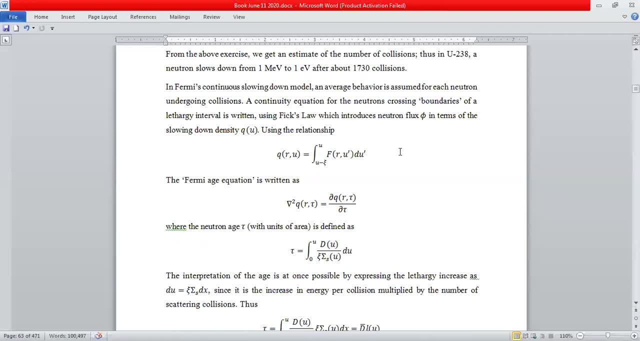 Now here: an average behavior, like I told you, is assumed for neutrons, So for each neutron undergoing collisions. So what Fermi did was he wrote a continuity equation for neutrons crossing boundaries of a leve прот corrugation interval. 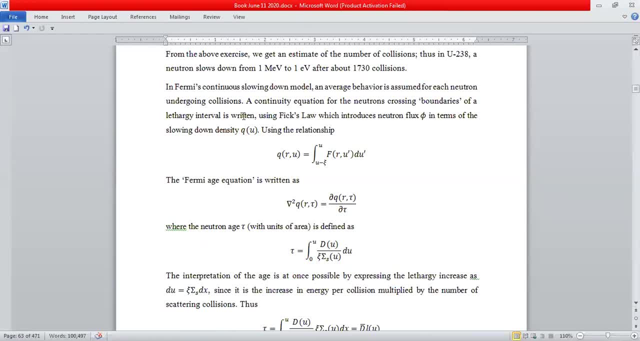 And remember I told you what's that? That's the slowing down density Q. So he wrote a continuity equation and used Fick's law. Fick's law is Fourier's law also. It's called Fick's law and it is called Fourier's law. 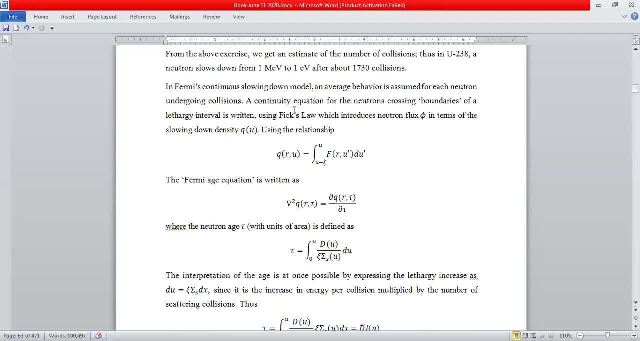 Cause side effect, Cause side effect, Cause side effect. And cause cause- Oh okay, is directly proportional to the negative of the gradient of the scalar cause. So there's a cause and there's an effect. So he said that the slowing down at a position r. 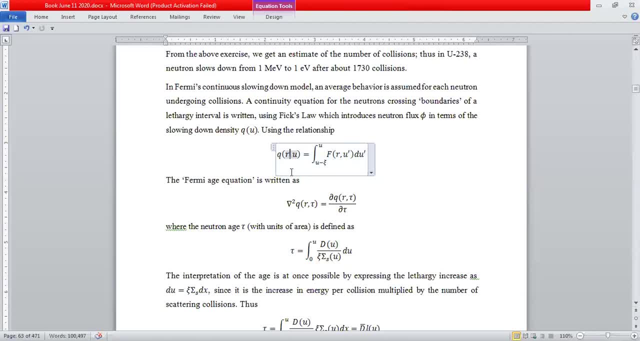 now, you see, we're not talking of an infinite medium, We're talking of a realistic room. So the slowing down density below a certain lethargy U, well, I should say below a certain energy E or above a certain lethargy U. 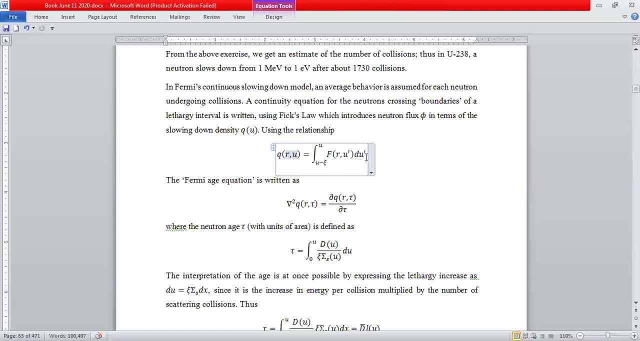 is the collision density, in that in some U prime which extends from U minus side all the way up to U, And if you do that, use Fick's law over here. So the first, the Fermi age equation he showed is del square. Q is dQ by d tau. 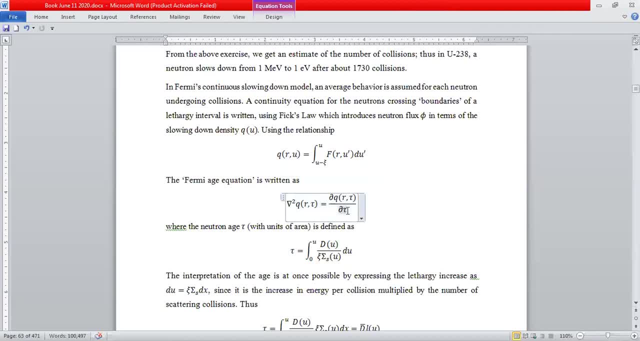 So there's something new over here. tau, It's not time, So, but it looks like a time dependent diffusion equation, doesn't it? So you've seen this before, but you haven't seen it here. You've seen in the time diffusion. 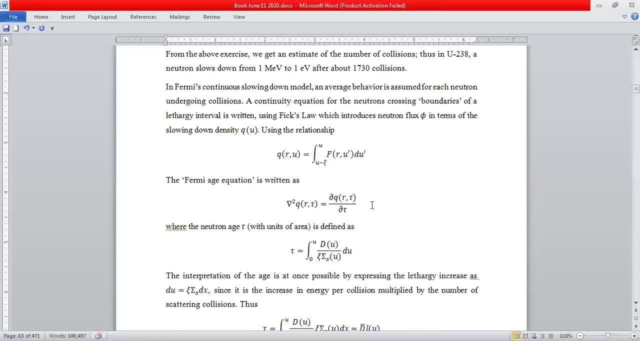 you've seen in the time dependence of concentration, for example of petrol or perfume. if you put it in a room, So the petrol or perfume would diffuse into the room, And if you're sitting far away from it, then after a certain while it reaches your nose and you start smelling the. 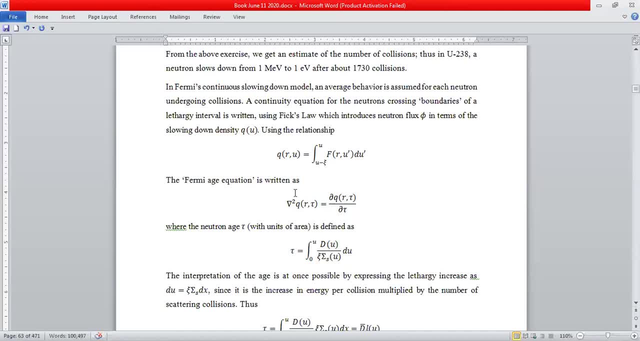 perfume or the petrol. This is that equation, but here it's for the slowing down, density Q, and it's called the Fermi age equation. Now, what is tau? Tau is a contribution by Fermi. He called it the neutron age. Now, age means time, right. 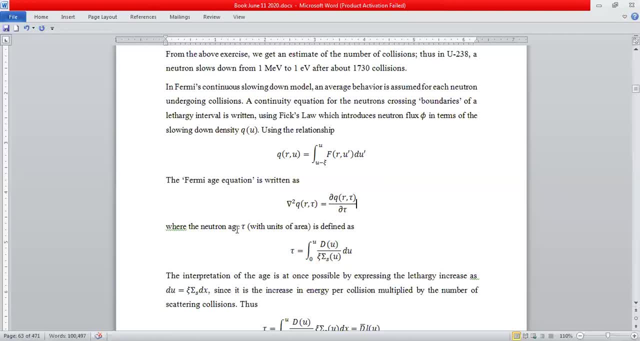 My age is so many years, Your age is so many years, but this is not an age in that sense. It's got units of centimeters squared, It's got units of area And from this derivation it's defined as the diffusion coefficient D. 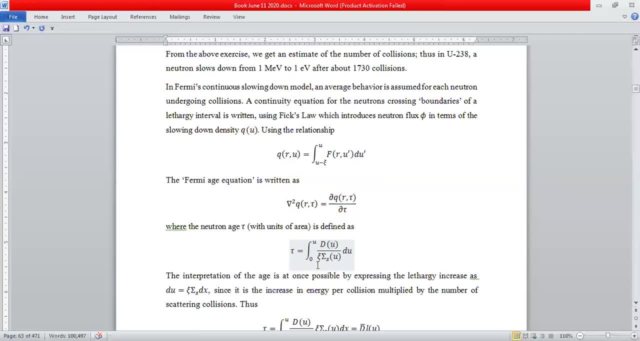 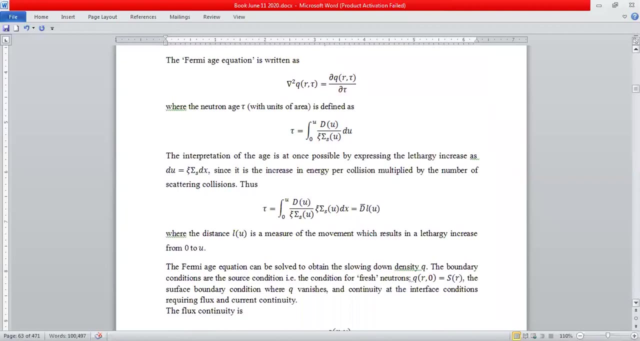 which comes out of Fick's law as a function of lethargy divided by excite, Sigma, S, U, D. So this is the neutron age, tau. The interpretation of the age is at once possible by expressing the lethargy increase as T. 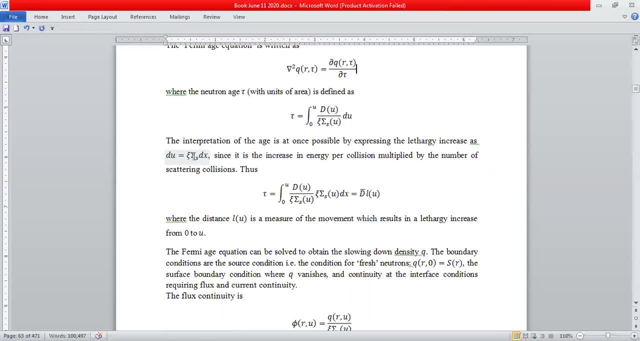 Now this is what happens in one collision: the lethargy increase. So if you multiply it by the number of collisions- Sigma, S, D, X- so you get the total lethargy increased to you. So so it is the increase in energy per. 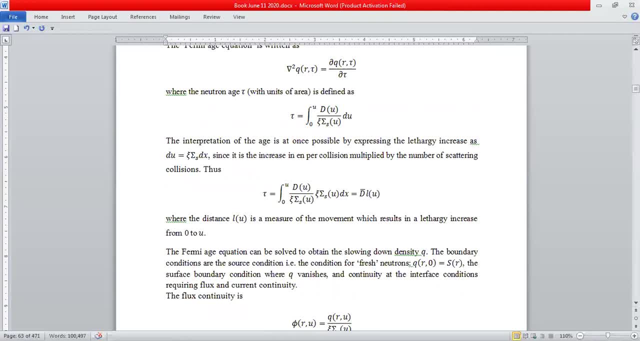 sorry, it is the increase in lethargy per collision multiplied by the number of scattering collisions. Thus the age is like this. The size Sigma S cancels over here. What are you left with? You're left with, if I take out an average value of the diffusion coefficient: 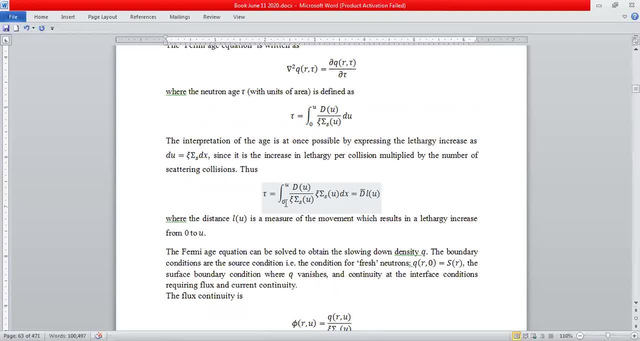 I'm left with the integral of DX extending from a lethargy of zero, meaning a source neutron, down to you, And let's say that it's a measure of the distance that you travel which results in an increase in a lethargy from. 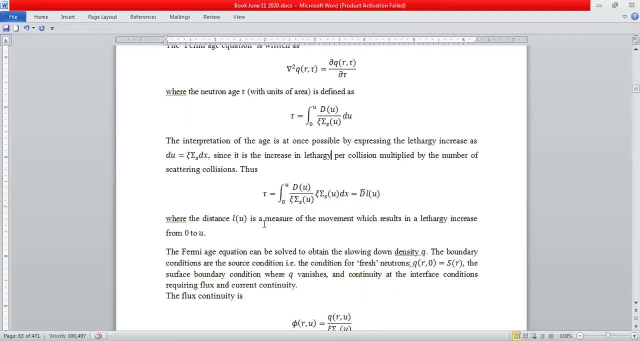 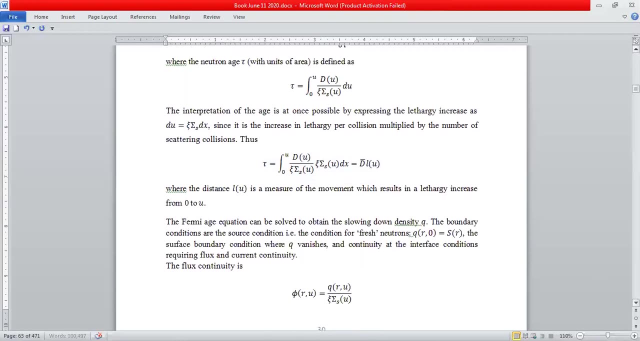 from zero to you. Now, what does this mean? It means that it is a measure. It means that age is a measure of how much area is covered area. I say area because, like a candle light goes in all directions, So it diffuses light diffuses. 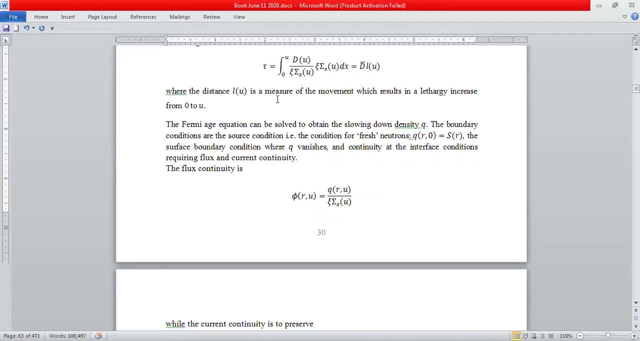 So jaw is D bar L? U, And this is the dist, where L? U is a distance. It's a measure of the movement which results in a lethargy increase from zero. to you, Such a powerful concept. Now, this is called. 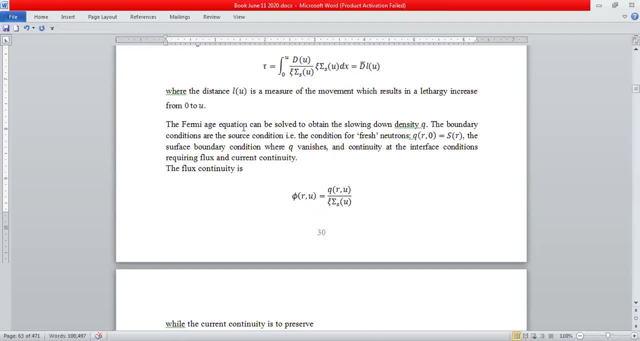 that was called the Fermi age equation for the slowing down density. It's an equation so you can solve it. It's got boundary conditions, The source condition. the source condition is for fresh neutrons which have zero age, which are just born. 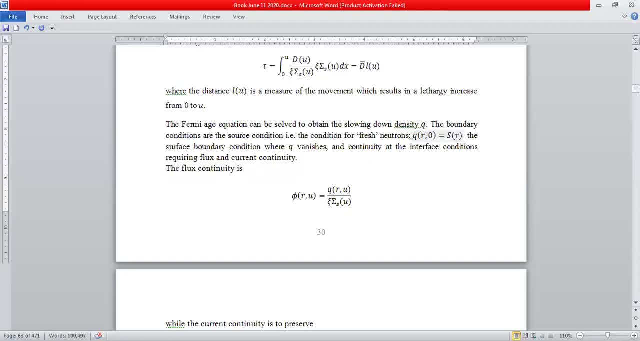 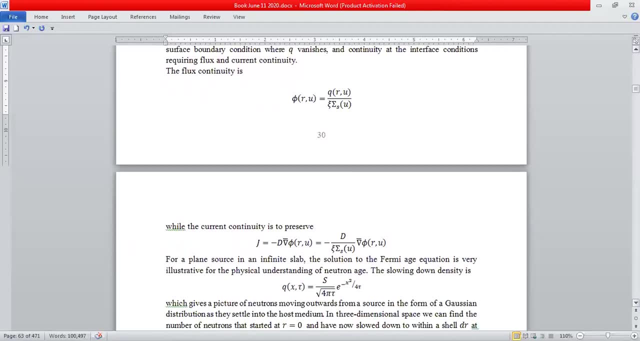 And which are those neutrons? Obviously the source neutral. So that's the source condition. What are the other two conditions? Well, they've got to be the flux and the current conditions. Now, remember I told you flux takes place in a volume element. 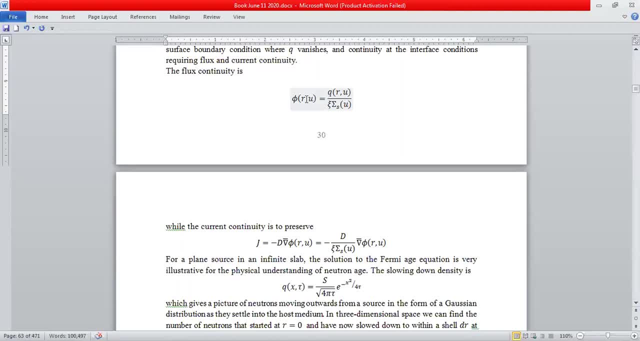 So flux is related to the slowing down density through fixed law And current is related to the flux through fixed law. So the flux continuity and current continuity translate into the continuity of the flux. So that's what you apply across an interface and you solve it. 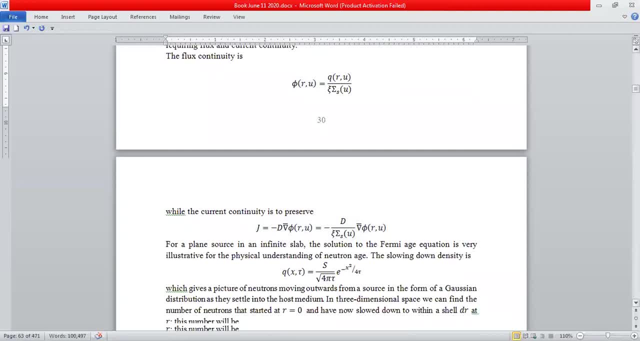 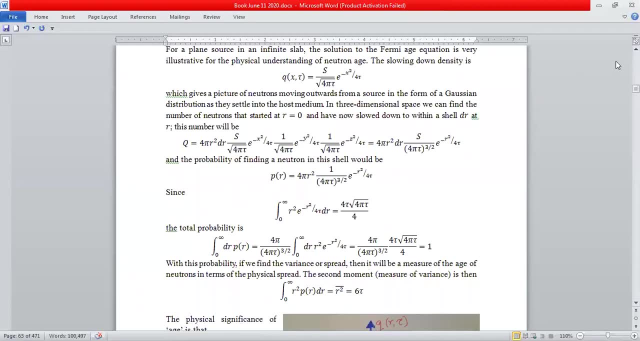 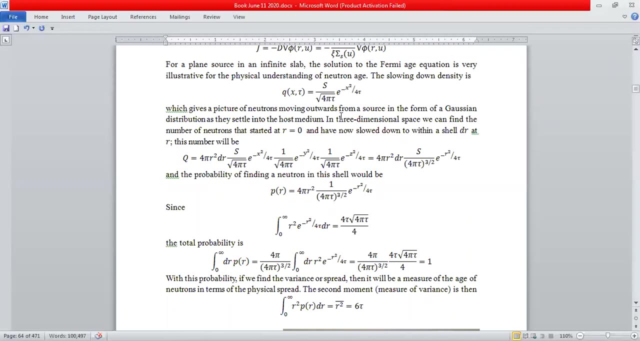 Now there are a number of possibility, possible configurations for which you can solve for me. for me is age equation. So let's look at a very simple one, because I'm trying to get you to a concept Now. a simple, a very simple elementary idealization is a plane source in an infinite slab. 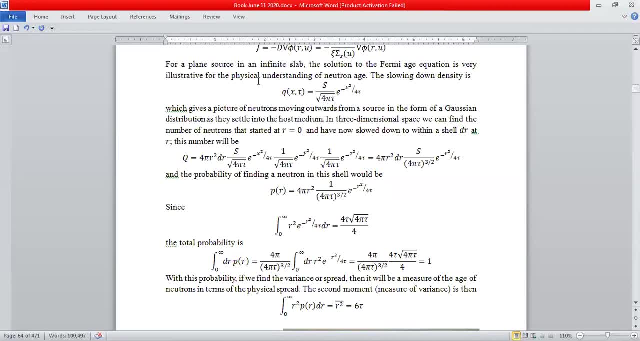 So plane, plane plane means a line in 3D. A plane is a, is is a surface, It's a wall. So a plane is the surface of a wall, which has an equation like: AX plus BY, plus CZ is equal to D, where ABC and D are constants. 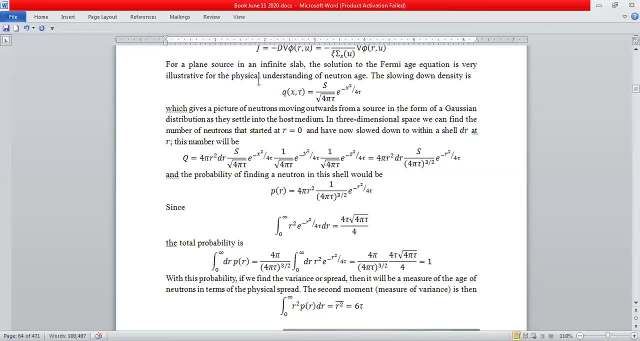 So if you have a plane source in an infinite time, freezing formula is an infinite slab. The slab slab means X. So if you take a plane source in an infinite slab, then the solution to the Fermi age equation is this: that to the slowing down density, 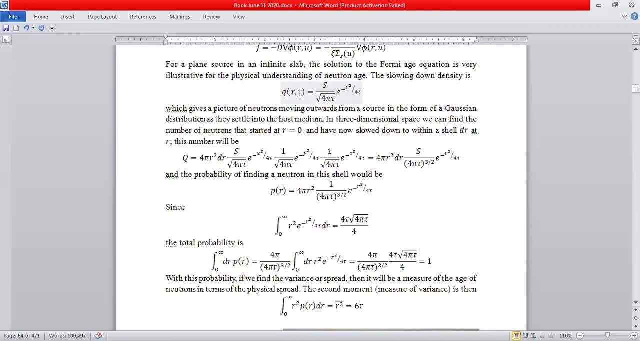 at the position X of a neutron that has a age. top is some constant times E to the minus X, square over two. I will see you later. Bye, photo. Now, I often wondered as a student. when I first read this it was Professor Mike Williams. 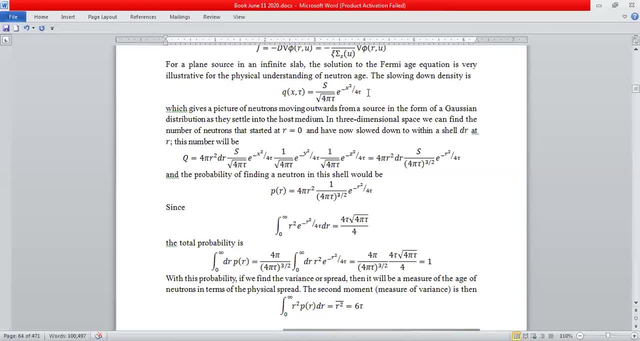 at Queen Mary College, from whom I first learned this, and in those days we didn't ask our professors questions They didn't like, and you know there was no such thing as a feedback or what you thought about a professor. A professor was an untouchable, too big. you're not supposed to ask questions. So 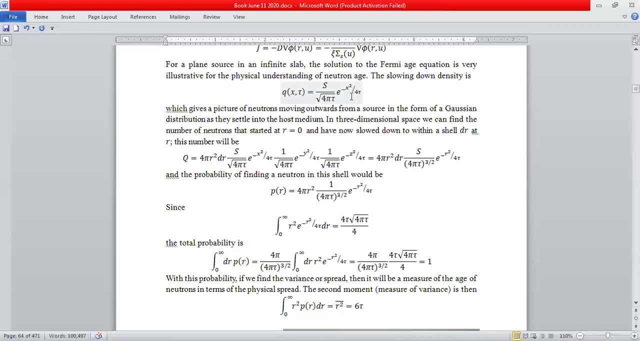 I didn't ask him this question, but what I wanted to ask, as a student, was that this looks like the time-dependent diffusion equation, and if I had asked him this, which you can ask me, I would say: yes, it is, because it's an exponential going down, dropping very rapidly: e to the minus x squared. 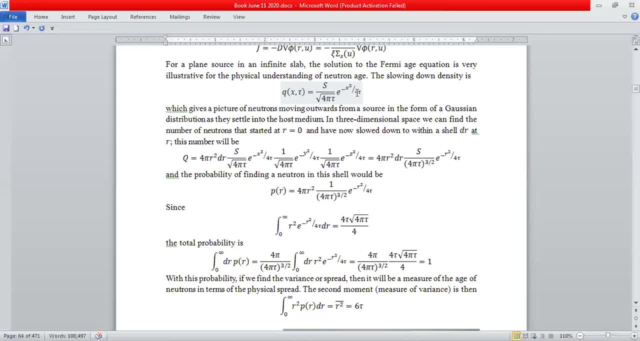 with a scaling factor 4 tau. and here the same photo appears in this form. So this is the slowing down density. Now, this is really good so, which means that I can stand somewhere near a source, a plane source, in an infinite slab. I can put my hand over there and 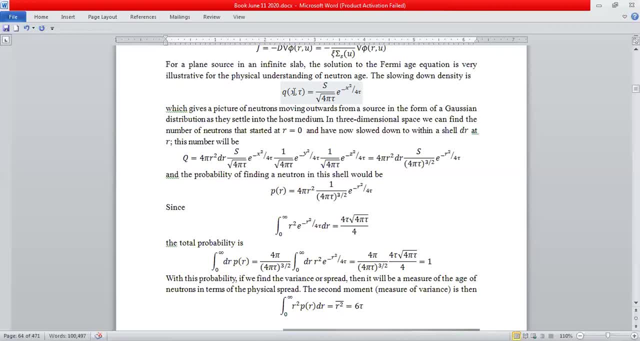 I can start counting the number of neutrons which are slowing down, which have, which have attained a certain age. Now, age is still not something which we've understood in this lecture so far, except that I've told you it's a measure. It's a measure of the movement, and 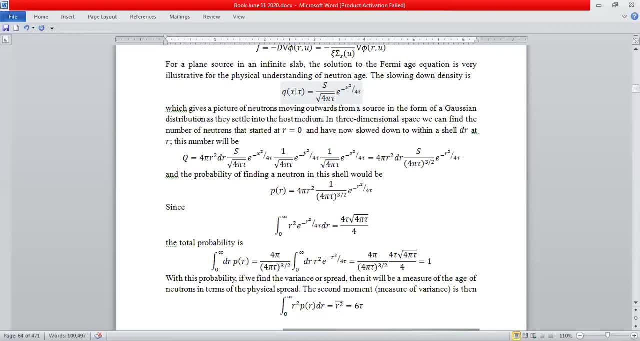 it's not time. It's got units of centimeters squared, but here is an expression for the slowing down density. Now I want you to make a picture of neutrons moving outwards from a source in the form of a normal Gaussian distribution, of a normal distribution, a Gaussian distribution, You know. 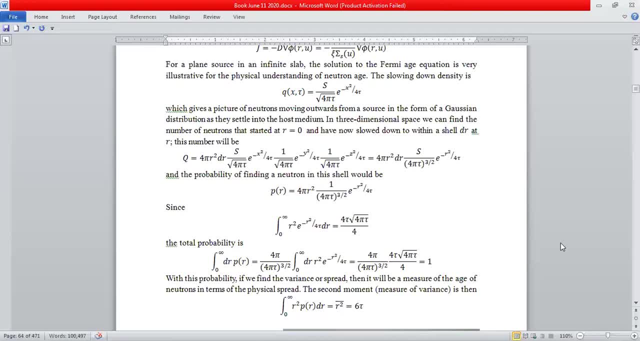 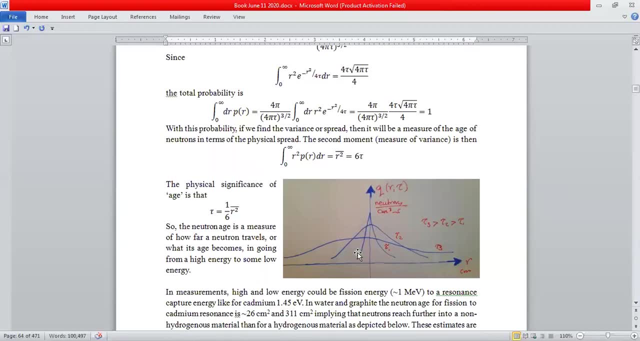 what a Gaussian distribution looks like. It comes down. So what I've done is I've made a little picture for you. This is a normal distribution, So something with an age zero. What was it? It's a delta function, and what is a delta function? 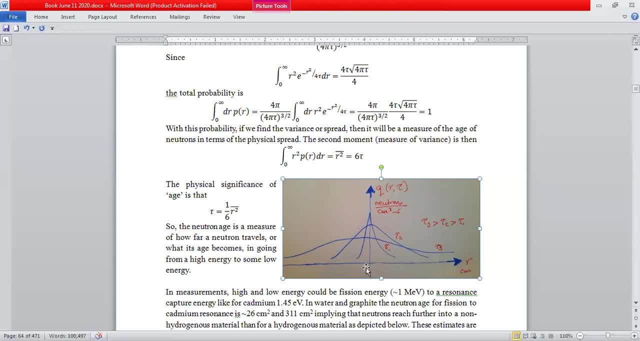 The Kronecker delta function. A delta function is a Gaussian which has zero width, which means it's on the y-axis. So that's the source condition that you put perfume in the room, you put neutrons in the room. they're just born, they have an age of zero, so they're on. 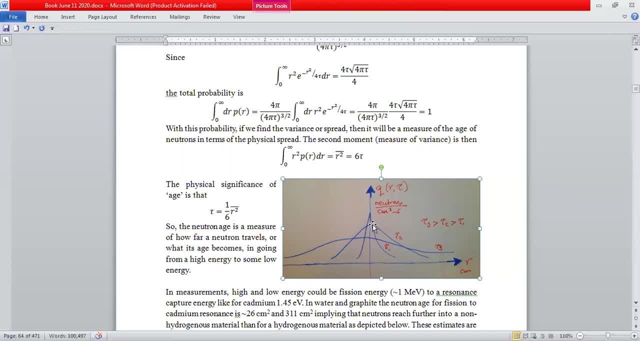 the y-axis, But after some time they've started diffusing. So look at what happens when a neutron reaches the age tau one: It's moved to some distance here and some distance here and tau is a measure of that movement. After a little while, when it's moved a little bit more, when it 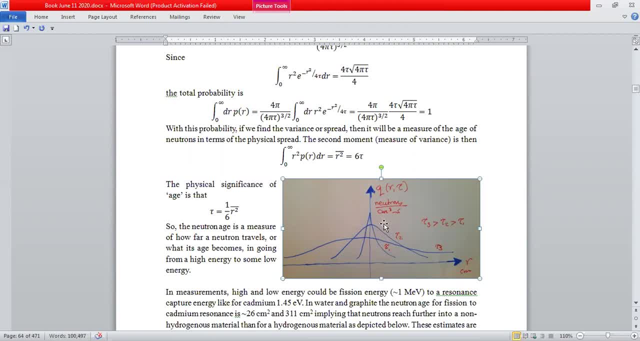 has reached the age tau two, then the Maxwellian, the Gaussian, the normal distribution has become a little bit wider, which means that it's extended further away into the room, further away from the source, when it was born as a normal distribution. So this is a normal distribution, This is a normal. 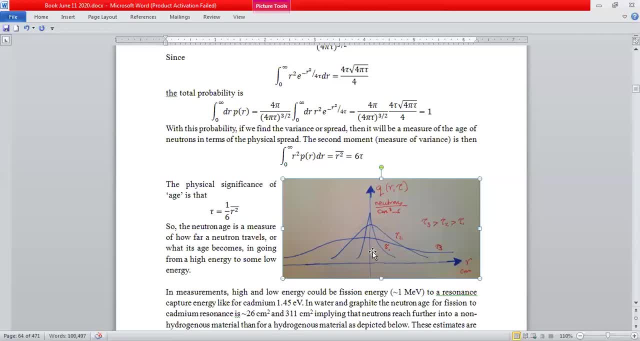 distribution. So this is a normal distribution. So this is an old neutron as a source neutron, which means that its age has increased. Now, when it becomes older, then my pictures are not very good. This should have been symmetric about the y-axis, so it becomes a more broader Maxwellian. 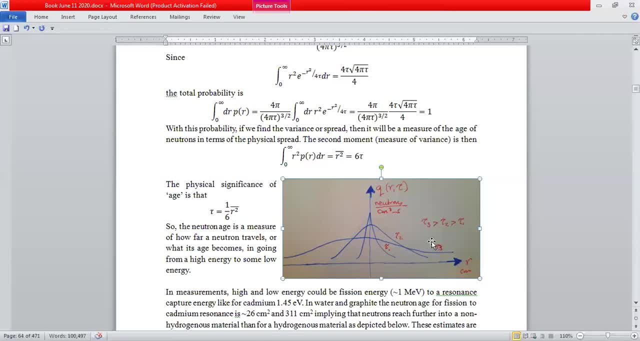 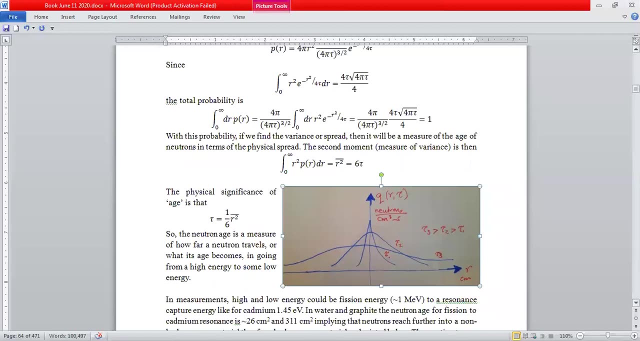 a broader distribution, a broader normal distribution. It's now an old neutron with tau three. So the age tau three is greater than age tau two is greater than the age tau. Now the. this shows you a plot of the slowing down. density versus R, and R square is X. 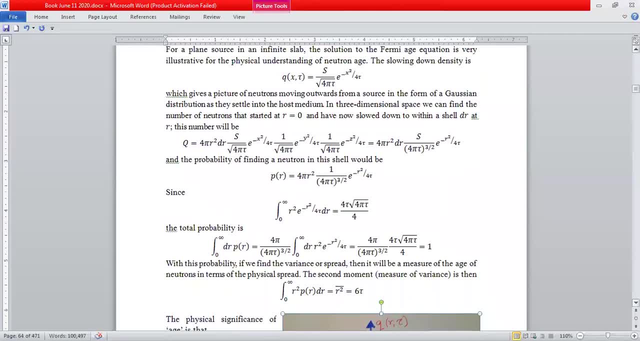 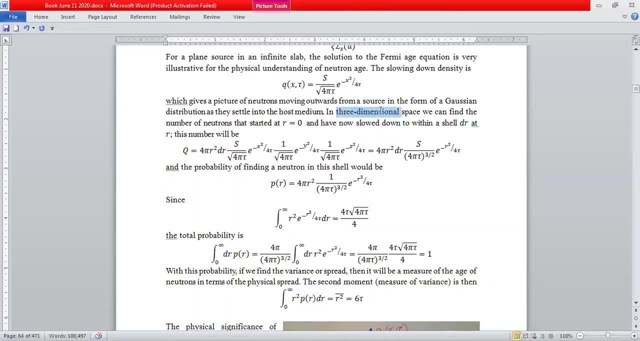 square plus Y square plus Z square. So if I extend this not only into X square, but if I extend this into 3D space for neutrons that started at R equal to 0 and now have attained some age, they have slowly moved down to within a shell. 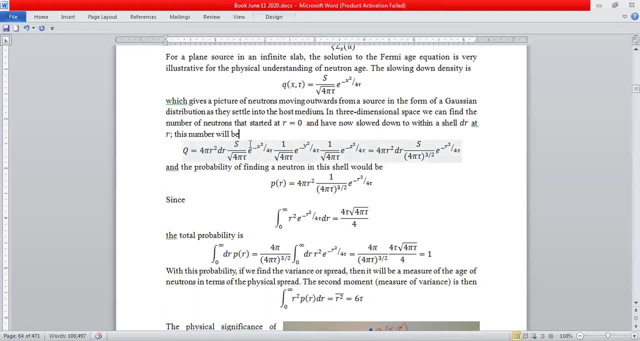 DR at R, So this number will be in the X direction, in the Y direction, in the Z direction. So I can write: X square plus Y square plus Z square is R square. So here's the volume element and this is the constant over here, which was a. 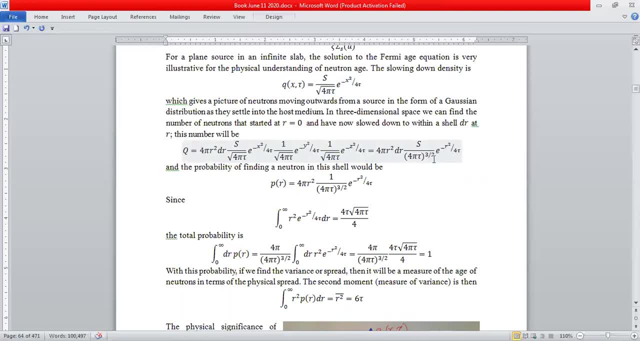 square root. now it's become to the power 3 over 2.. So this is a fascinating thing, and so the number of neutrons I've written as capital Q. So this is a fascinating thing, and so the number of neutrons I've written as capital Q. 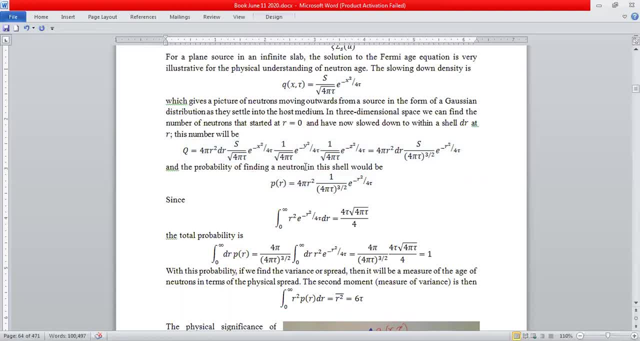 So the probability of finding a neutron in this shell would be PR. So PR would be: if I take the DR out of here, so and the DR out of here, so I get a probability. Now, whenever somebody tells you this is a probability, the first thing you should. 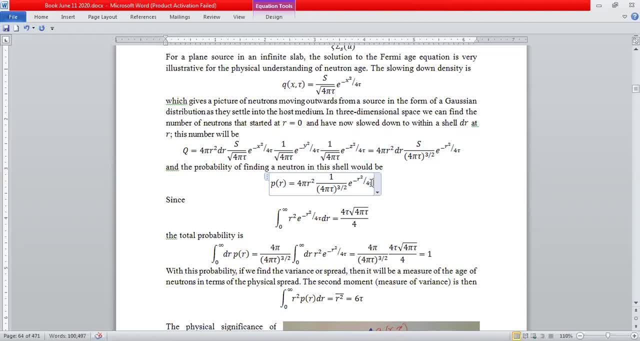 ask them to do, or the first thing you should do yourself, is to show that it integrates to one, because if you cannot do that, then of course it's not a probability. So the first thing I would like to show you is that if you integrate to one, then of course it's not a probability. So the first thing I would like you to do is to show me that it integrates to one. 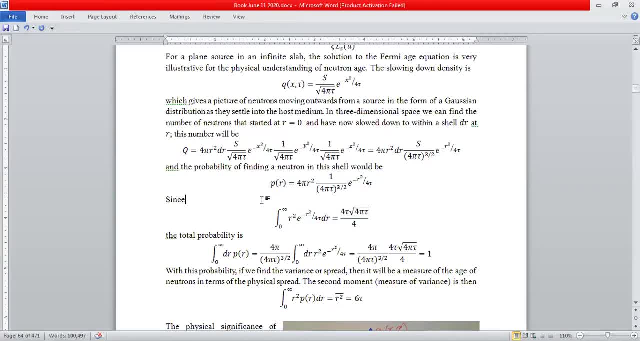 Well, I did that for you. so because I have not been satisfied myself. so I wrote this probability like this and I looked at this integral and this integral comes out to be the force cancel out tau times square root of 4 pi over tau. So the total: 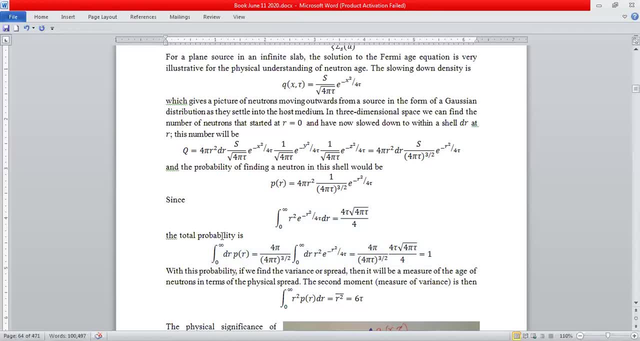 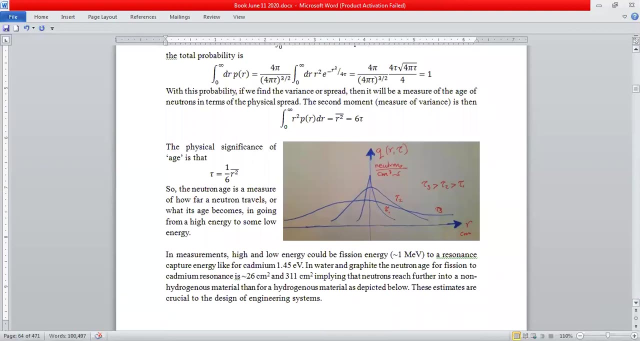 probability. if I look at the whole of space from R equal to 0 to infinity, well, it doesn't matter, It does come out to 1, so I'm really happy about that. So I'm really happy about that. So what I'm telling you is correct. Okay, now, once we've got the probability, what? 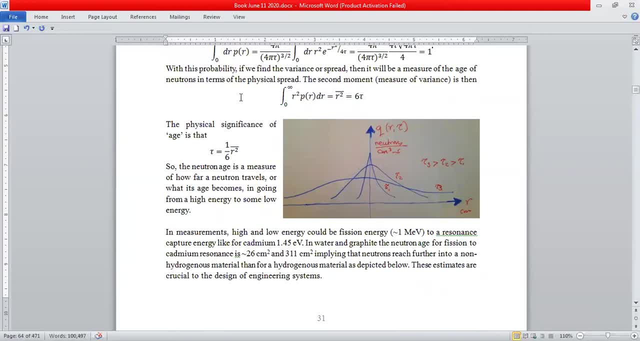 do we do? We look for the second moment because we want to know what is the age. So the second moment of anything, any distribution function, is its variance. It's a measure of its spread, and that's precisely what the age of neutrons is. It's a spread. So the second moment is: 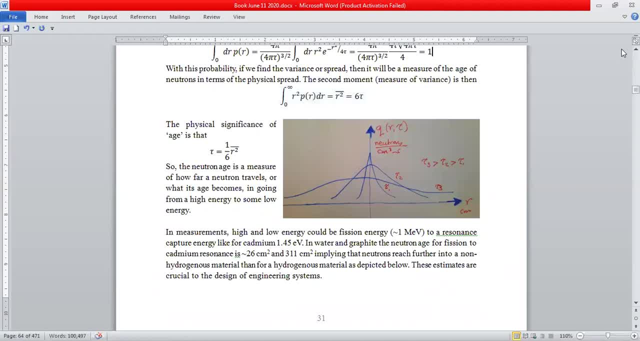 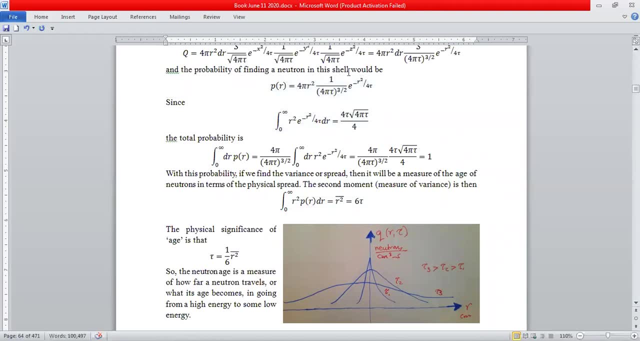 the R square times P? R. Now the P? R already has an R square, so this integral becomes R to the 4.. It becomes 4 pi R to the 4 times all this. When you integrate this, then, and that's the average value of R square by 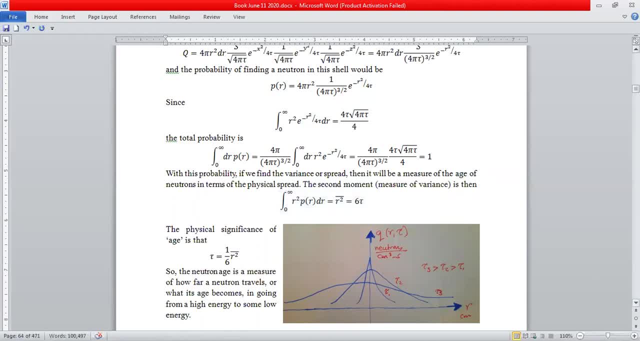 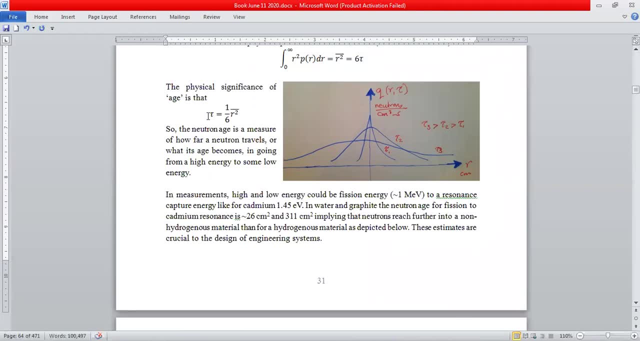 definition and it comes out to be 6 tau. Isn't that beautiful. So so I now have a result that tau is 1 sixth of the spread of neutrons of age, tau, which started off as fresh neutrons from a source where the age was 0. Now that's. 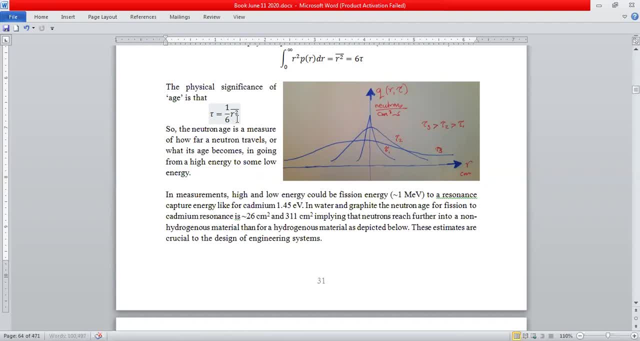 beautiful. That shows you neutrons slowing down. So so the neutron age is a measure of how far a neutron travels or what its age becomes In going from a high energy neutron to a lower energy neutron. Okay, again, this is such an important picture which I've got for you over here that it's a normal. 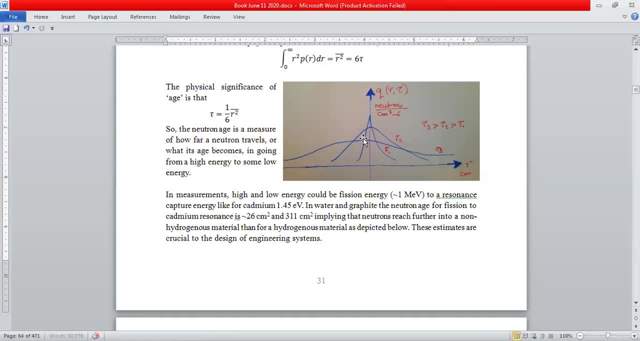 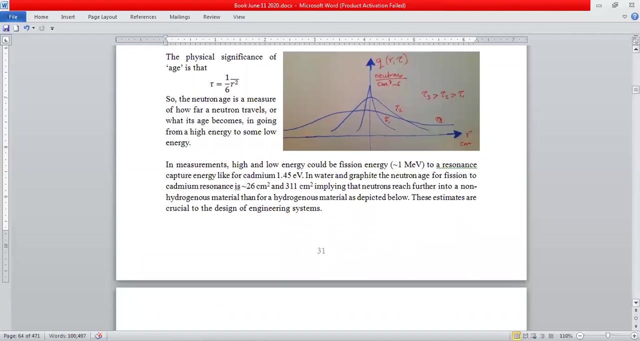 distribution. It makes sense. This is our perfume: diffuses in a room. This is our petrol: diffuses in a room. and this is exactly how neutrons diffuse from high energies to moderating energies. Okay, now let's convert that into practical something. You're an engineer. You want to design something. You want to. 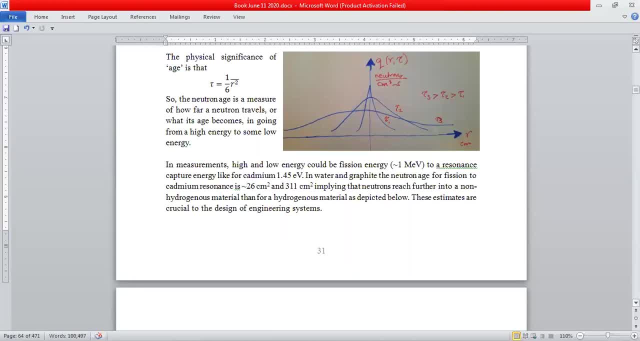 tell somebody, it's 2 meters wide, 3 meters high, It's a cylinder surrounded by this, and up is that material and down is that material. So, so, what can you say from the neutron age? What good is it? Well, it, first of all, it gave you a concept. 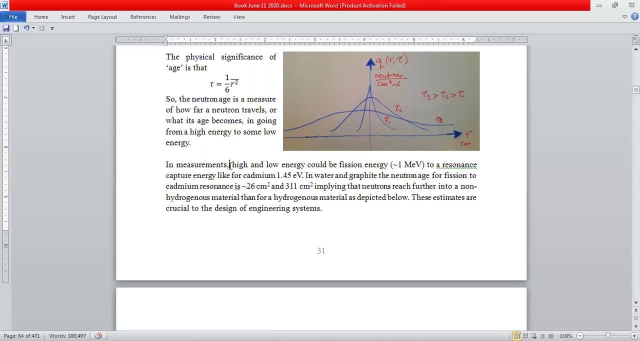 Now in measurements. so what a scientist gave us. that an engineer went to the lab he tried to measure it. he or she tried to measure it and I told you that they took a sheet of a little foil of cadmium. Cadmium captures everything at 1.45 eV. 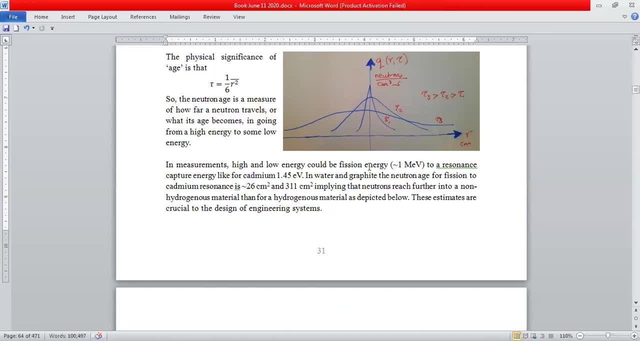 So it bombarded this cadmium strip with the flux of fission neutrons, which had such a high energy of millions of electron volts, capture it in cadmium to its resonance, and measured the time taken and how far the distance was, and measured the slowing down. 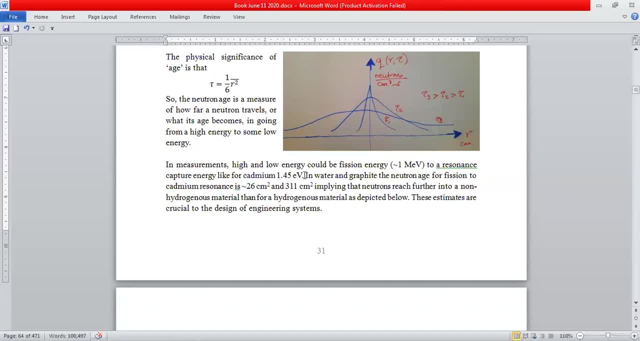 density and said: is it correct? is the Fermi age equation correct? does it give you a proper prediction of what things are? so when they measured this for water, they found that the age is approximately 26 centimeters square. but they measured it for graphite and they found the neutron age was 311 centimeters square. 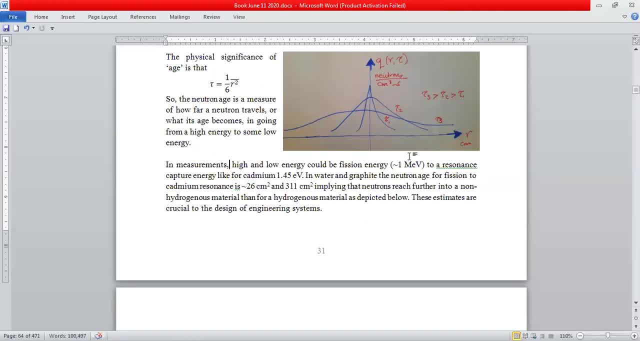 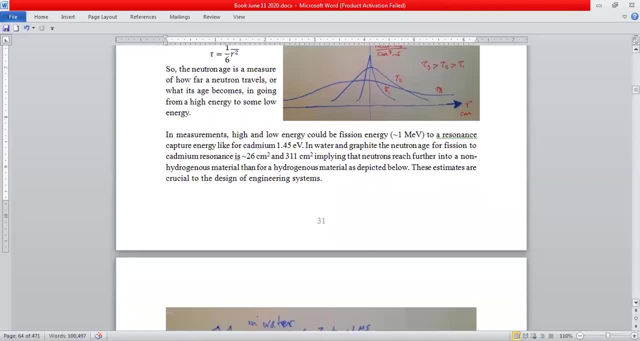 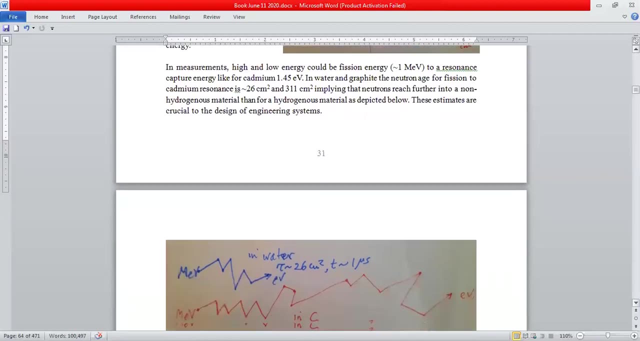 but from this energy to this energy, so from about. so it depends on what your starting energies and what you're capturing on, so this can give you. the neutron is now what? what does 26 centimeters square mean? what does 311 centimeters square? let's look at, and this is what it means, that let's make a. 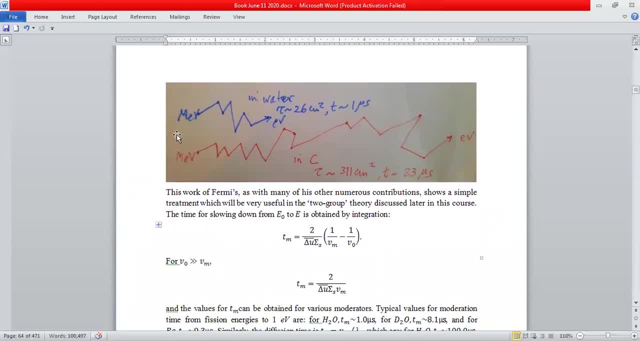 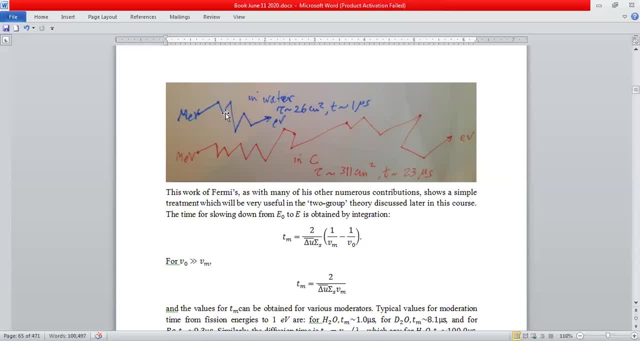 now it's journey from MeV to Evie. all these collisions took it through a cross-sectional area- 26 centimeters. now if I take the square root of that, that, I'll get centimeters. so what if I tell you that it traveled roughly 5 centimeters from the source? so make a picture in your mind of a jug of. 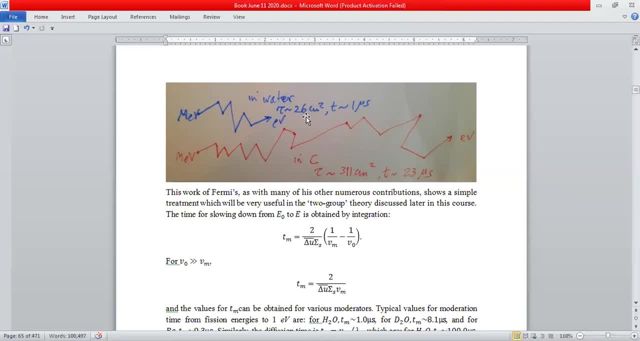 water, or or a bigger bucket of water and you put a neutron source in there, and if the bucket of water is 24 centimeters centimeter radius, then between 0 and 20 centimeter it must have gone through five of these neutron ages. right, and how much time did it take? now I'll just show. 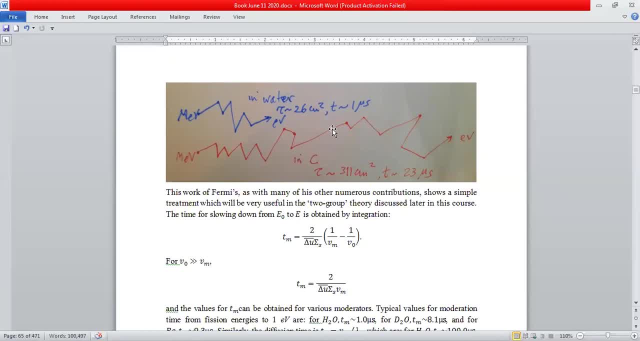 you how we can estimate the time from the Fermi age equation? so in water it goes like that. now, what about graphite? so in graphite, the same fission, neutron, MEV, the red path. it went here. it collided with a graphite carbon atom, went here, here, here here, losing energy. of course the alpha is a little bit. 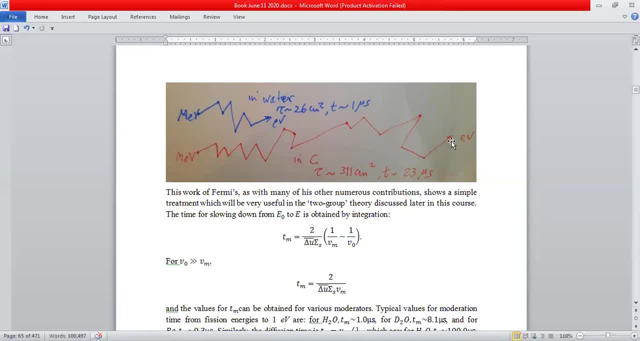 higher than it was for hydrogen. it goes here and all the way here it becomes an EV, ELEV, EV neutral. so see, this distance is much bigger than this distance. so, if you want to think of it this way, so this is about 5 centimeters. and what's the? 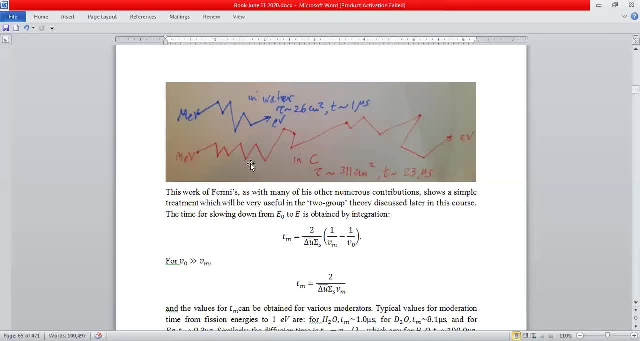 square root of 300. so it's a square root of 300. so it's a square root of 300. so it's a about 17.. So let's say it's 17 centimeters, So 5, 17.. So what does it tell you About? 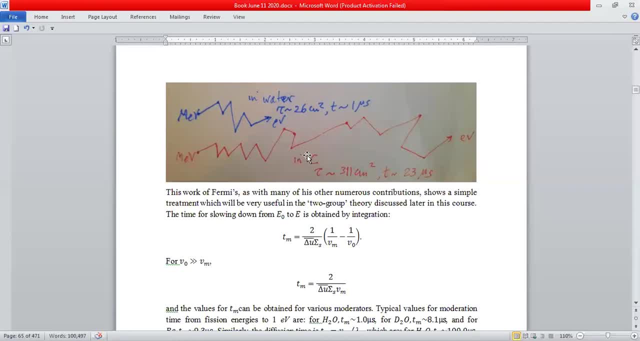 three times. So as an engineer, what I say is that slowing down or neutron age, is about three times more in graphite than it is in water. So if you ask me to design a nuclear reactor, so I already know what kind of dimensions to use, So I can tell you how much distance. 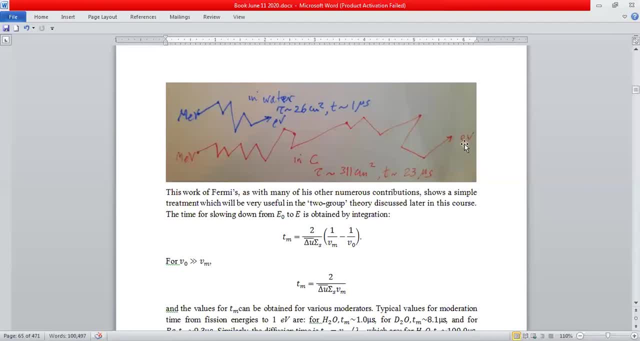 it's going to be for me to come down to some good energy if I want a thermal reactor Now, I haven't told you that it's going to take one hour. Is it going to take you a second, a millisecond, a microsecond, a nanosecond? So how much time will it take? Do I have to? 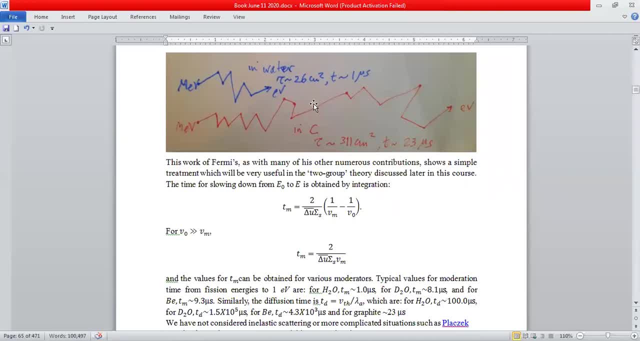 keep waiting till tomorrow for one MeV neutron to become a one Ev neutron. So this work of Fermi's, as with many of his other numerous contributions, you can go through Fermi's works. You'll be fascinated with him. a genius of his times died at the age of 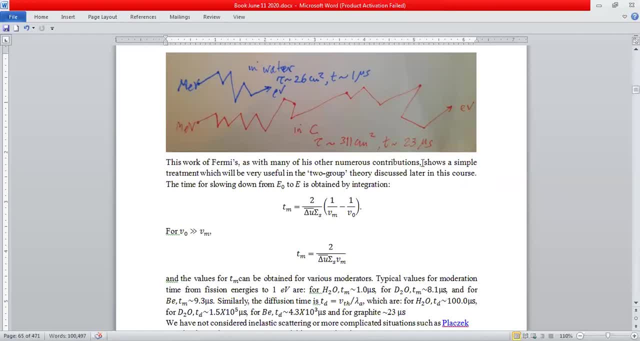 52. He was an Italian, started from a university in Pisa, Then he went to the Manhattan Project in America And in the first nuclear weapon test it said- I remember that as a student, I think- my professor, Professor William probably, if I'm not mistaken- he said he was an outstanding. 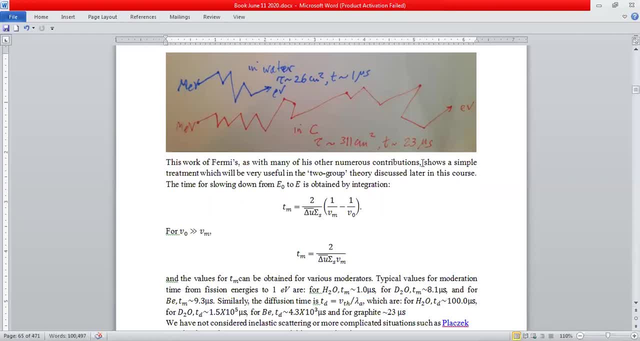 person for me. He put an envelope over there and from the force that he felt on the envelope he said: this is a 20 kiloton nuclear weapon. So that was his genius. He tied day-to-day life with such difficult things And what you just learned, the Fermi age equation, is one of. 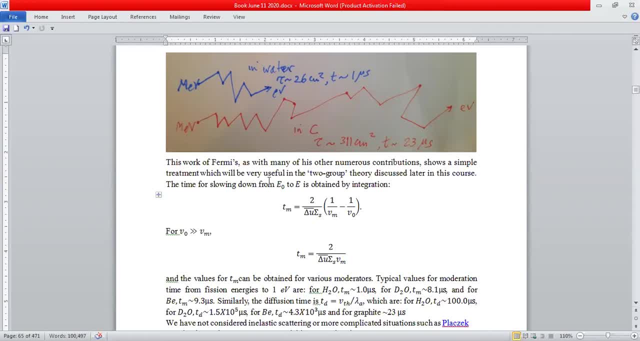 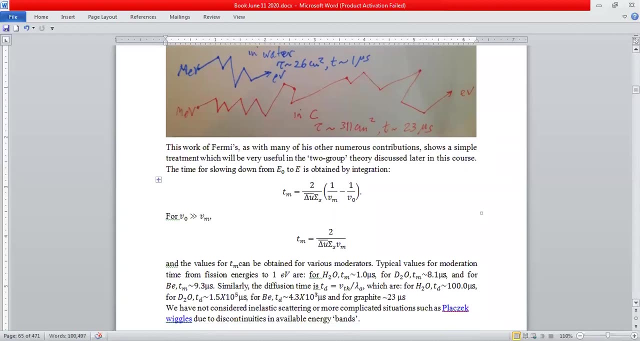 those contributions of this. So this shows a treatment which I will carry forward, and we all do this when we learn how to design nuclear reactors from starting from very simple two group theory, two energy group theory. So how much time does it take Now if you know how? 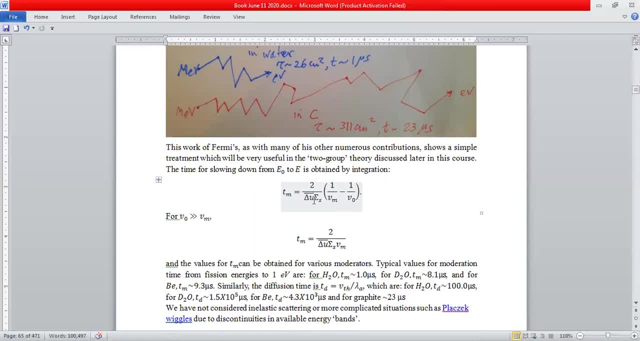 much lethargy you gain per collision and you know how lethargy is related to energy. So you can say that the number of collisions you also know. So you can write this down in terms of energy, You can integrate it from some source. energy E naught. at which it's, at which its speed was V naught. 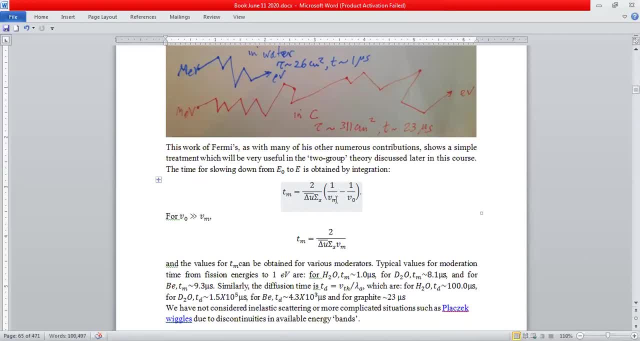 Down to some energy, EM, at which the speed of the neutron was VM, And here you get a moderation time If your source energy is much greater than your moderating energy, which of course here it is, because it's one MEV and one EV, So it's a million times more, So I can just throw this term away. 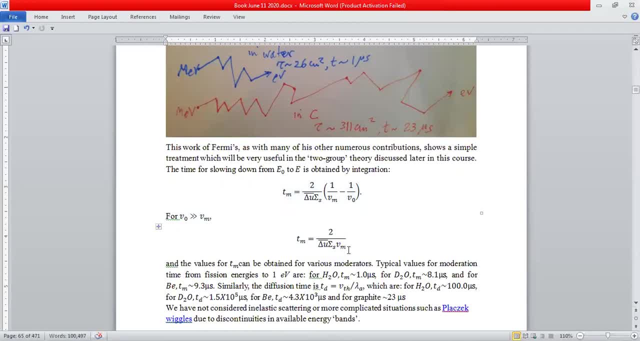 because 10 to the minus six, and this is one. So I get a beautiful expression for the moderating time. Now for water. if you look at the water, you can see that it's 10 to the minus six, and this is one. 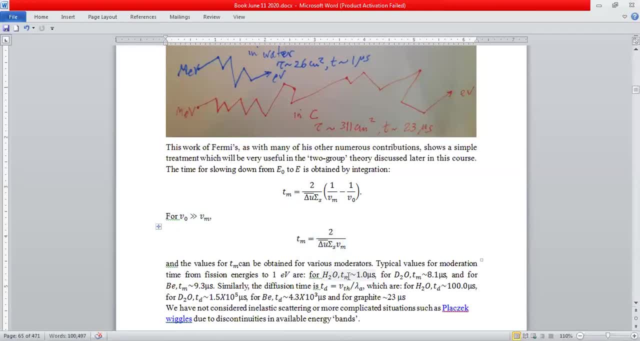 Now for water. if you look at the water, you can see that it's 10 to the minus six and this is one. So if you put these values in, you get about one microsecond For heavy water, for light water, 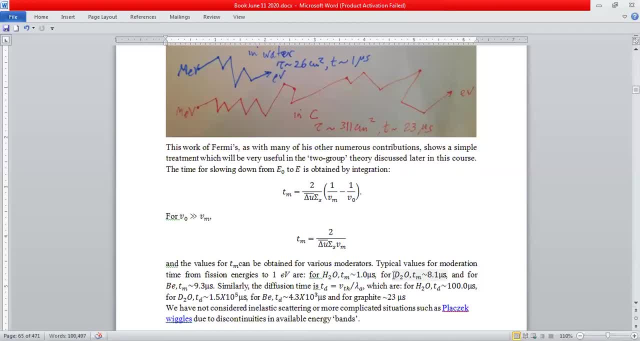 you get a microsecond heavy water. Now what's the heavy water nuclear reactor? It's the Canadian deuterium uranium CANDU reactor. So a light water reactor has a moderating time of one microsecond, whereas a heavy water reactor using deuterium D2O water- heavy water- has a moderate. 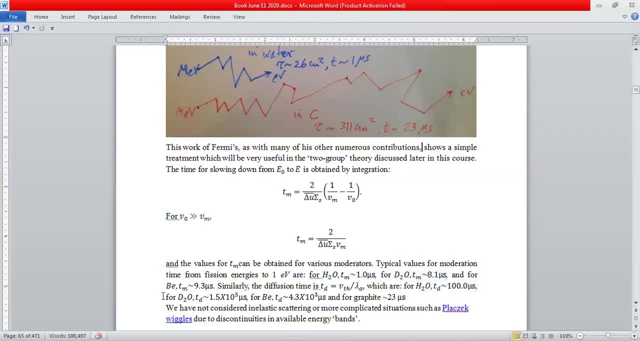 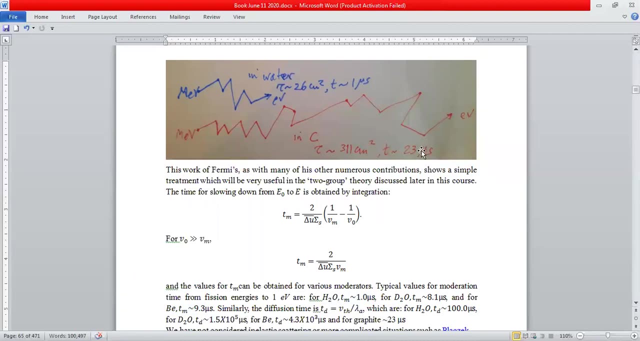 rating time about eight times that. And beryllium, which is used as a reflector, has a moderating time of 9.3 microseconds. Graphite has about 23 microseconds, So look again at this picture. So I don't have to wait till tomorrow. I have to wait microseconds, and I don't even know how small. 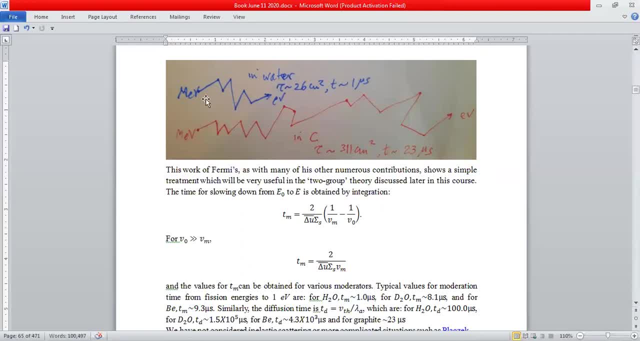 a microsecond is. I can't feel a microsecond. So neutrons are really fast. So a 1 million electron volt neutron slows down. So it's a million electron volt neutron. So a one million electron volt neutron slows down to a one electron volt neutron by traveling an area of about a spread of 26 centimeters square. 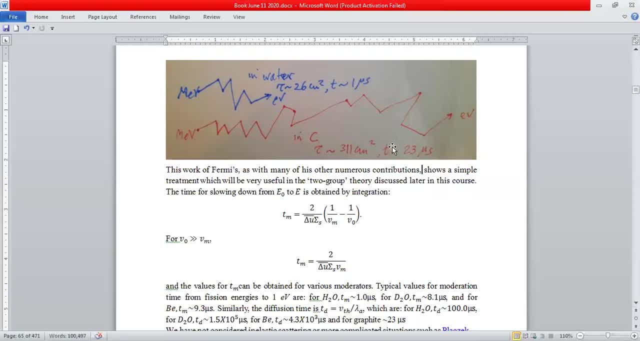 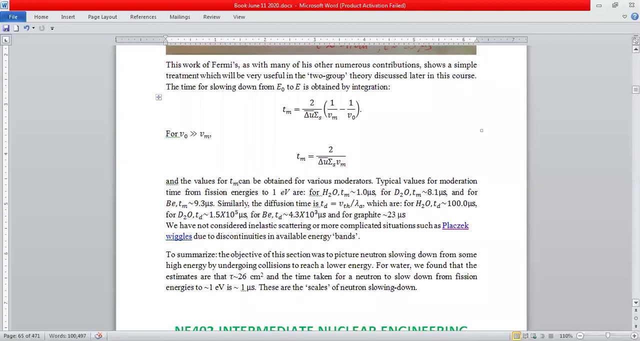 It does all that in one microsecond And in graphite it takes 20 times, 23 times more time than that in water And it travels a much greater distance. So this is what I wanted to tell you about the slowing down process Now. 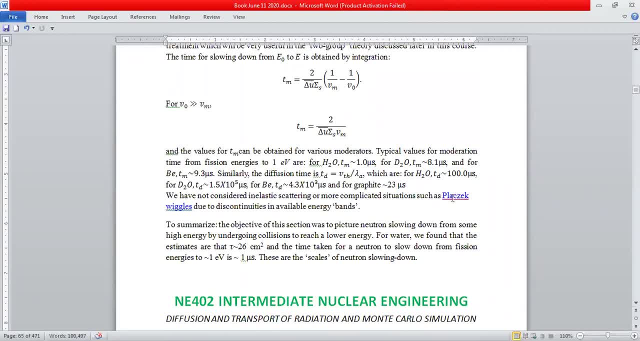 the Plachek-Wiggles. I did not discuss in detail, but you can go to this paper that you're seeing over here on this link, And I'm sure this link will be in the recorded version. I'm doing this on Zoom So you can go on this paper. This is a very old paper because this work was done as I 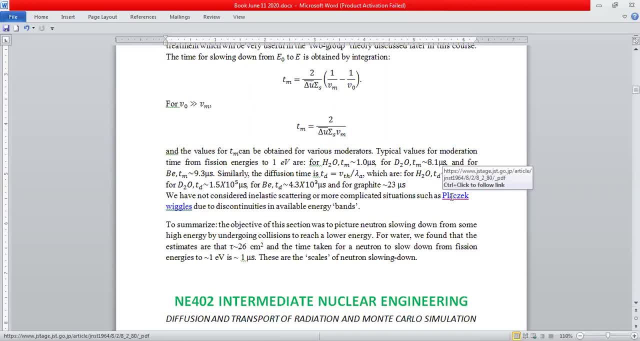 told you in the 60s and 70s. These days we don't use Plachek-Wiggles very much. The mathematics was really fabulous in those days. But it's a very good paper. It's a very good paper. It's a very good paper. 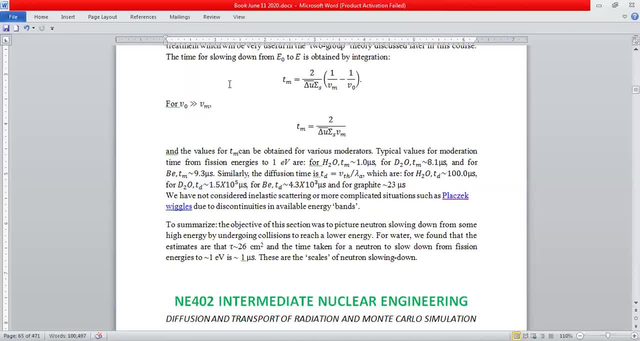 After all these days, now we've got computers, So later on in this course I'll tell you how you can do all these things and much more, using Monte Carlo simulation. To summarize what did we do in today's lecture, The objective of this section. 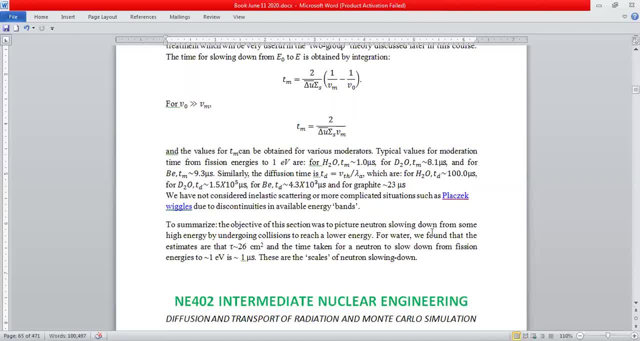 was to make a picture in your mind of a neutron slowing down from some high energy by undergoing collisions to reach a lower energy For water. we found the estimates are from 1 MeV to 1 EV of neutron age of about 26 centimeters square, The time taken from fission down to about one eV.